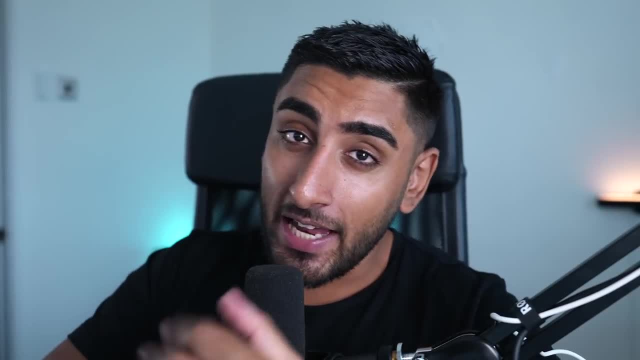 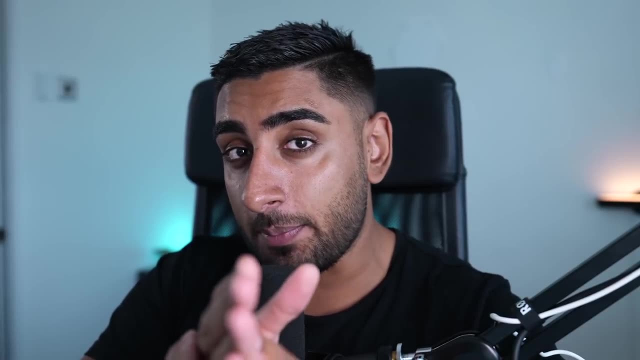 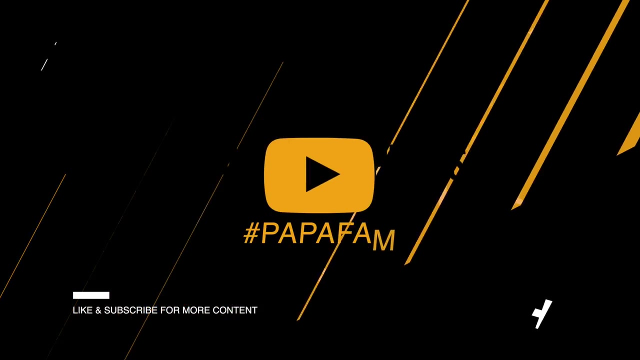 Yo, what's going on? Puppet Fam, Welcome back to another video. Today we're going to learn all about props, Why they're so crucial to you mastering it as a React developer. Get ready, roll the intro, let's go. So today's video is made possible by the amazing guys over at Skillshare. 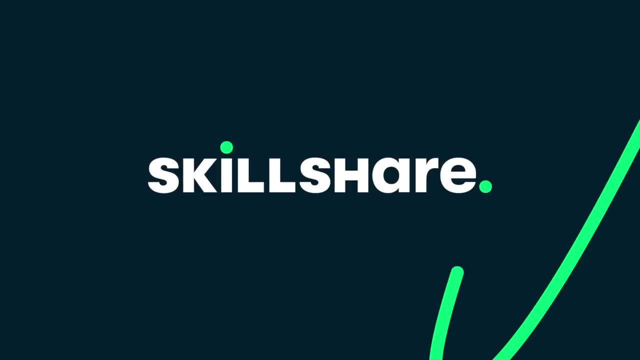 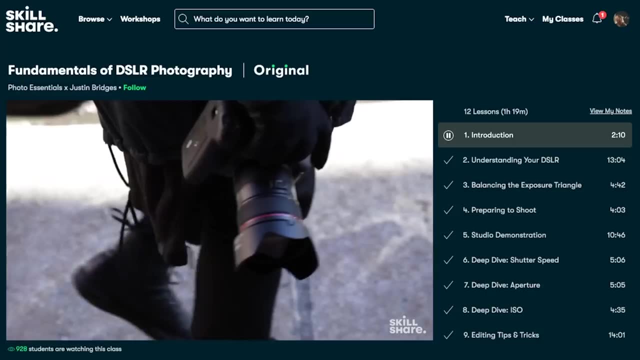 Before we get started check this out. Skillshare is an online learning community where millions of people come together to take the next step in their creative journey. The thing I love about Skillshare is that there are no ads. They're always launching new premium classes and they 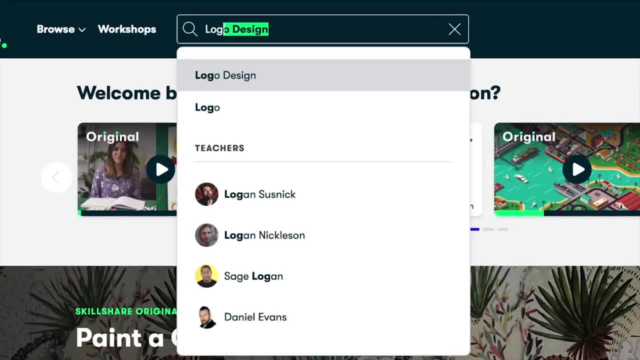 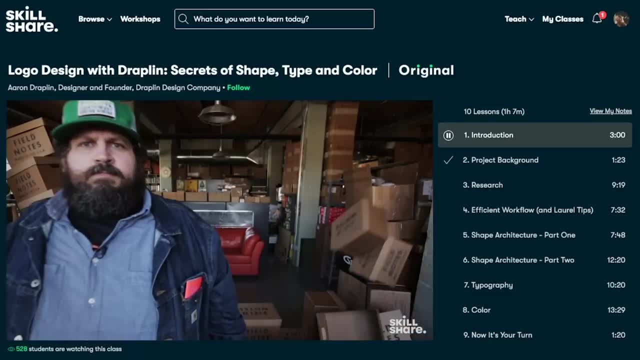 also recommend really interesting classes. So, before you know it, I'm actually no longer watching TV or Netflix. All I do is watch Skillshare while I'm actually eating my food. Most classes are under 60 minutes, so they should be able to fit any schedule, whether you're super busy or you've. 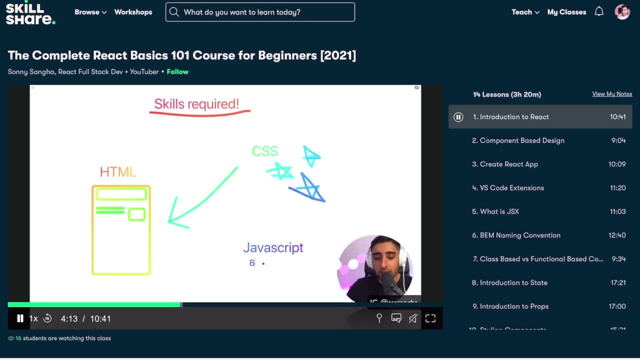 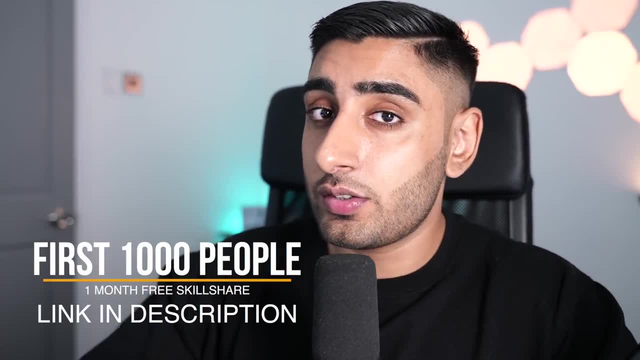 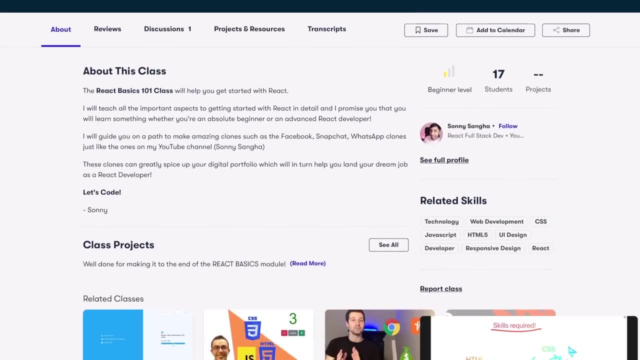 got a little bit more time on your hands. I've actually gone ahead and dropped the React Basics 101 entire class on Skillshare. The first 1,000 people to use the link in the description are going to get a free month worth of premium Skillshare and you're going to be able to, with that, access the React Basics which I've 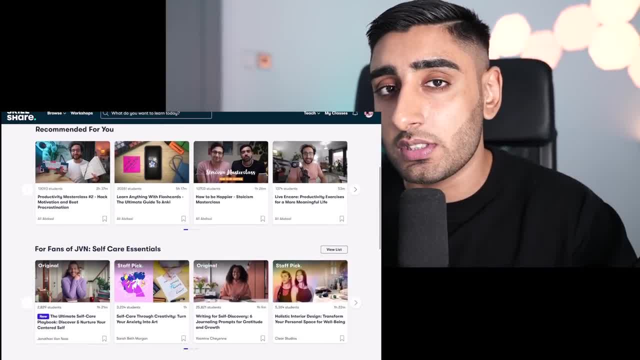 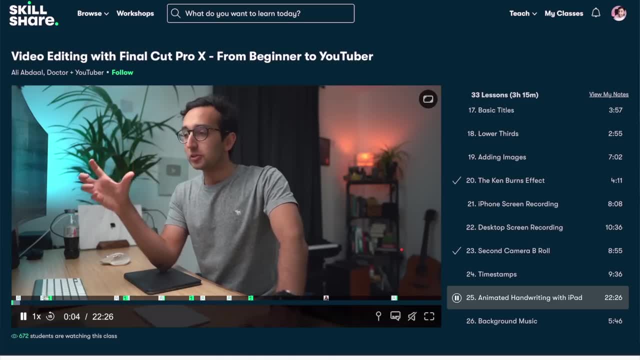 uploaded. On top of that, you're going to get access to thousands and thousands of courses available on Skillshare's platform. I've actually been checking out an amazing video editing class at the moment by Ali Abdaal, where I was actually able to find out how I could use my iPad to add. 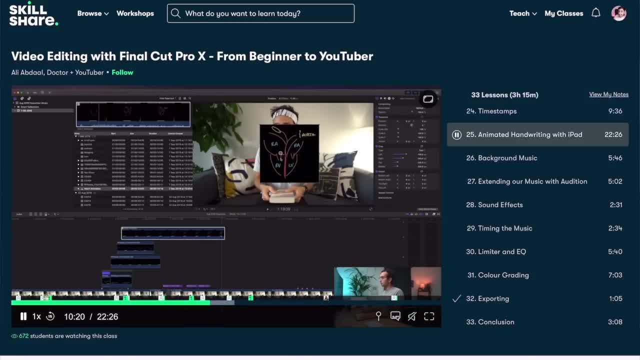 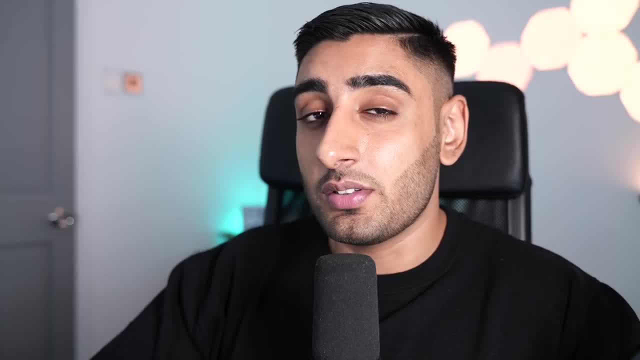 animated handwriting into my videos to level up my production value, And now I'm making the best use out of my iPad as well as leveling up my Final Cut production game. So this is just an example of the amazing value that I've got since I've signed up at Skillshare. 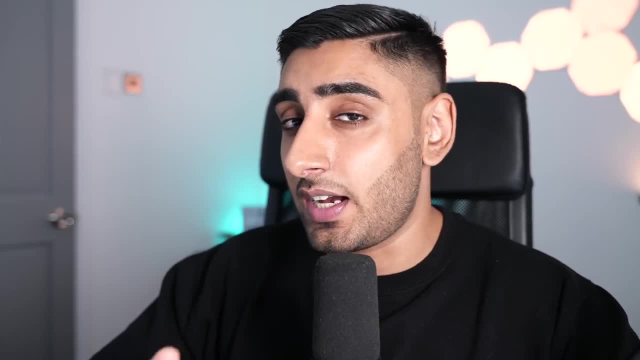 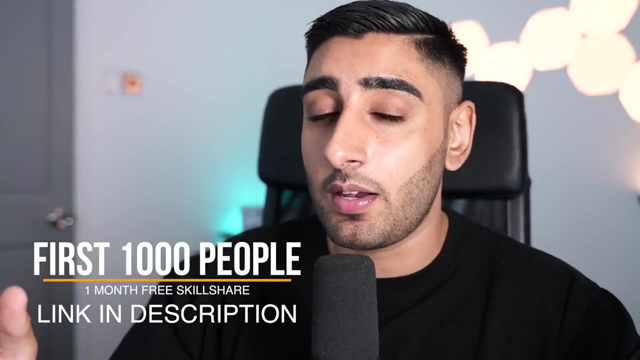 And if you guys want to go ahead and benefit from this, just like I have, then go ahead and remember: the first 1,000 people to go ahead and grab that link are going to get one free month of Skillshare premium, which means that you can access my React Basics 101 class. It's completely free, You have. 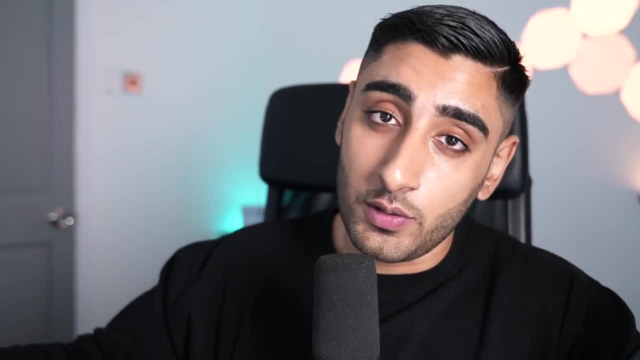 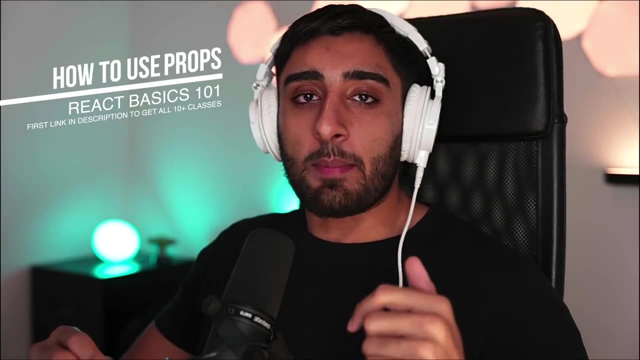 nothing to lose, And then after that you can go ahead and continue. if you're enjoying what you see on Skillshare, What's going on, guys? Welcome back to another lesson. In today's lesson we're going to be talking about props. 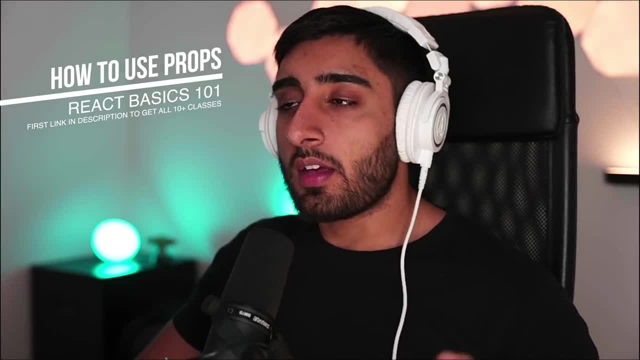 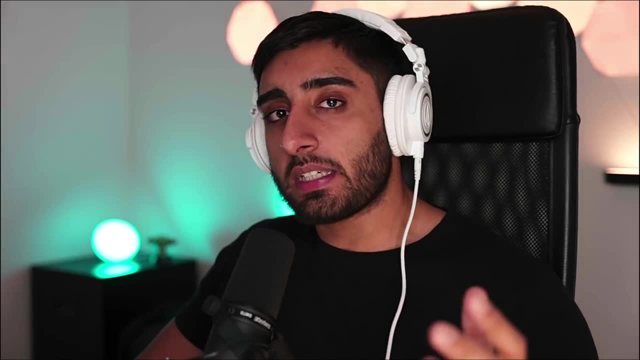 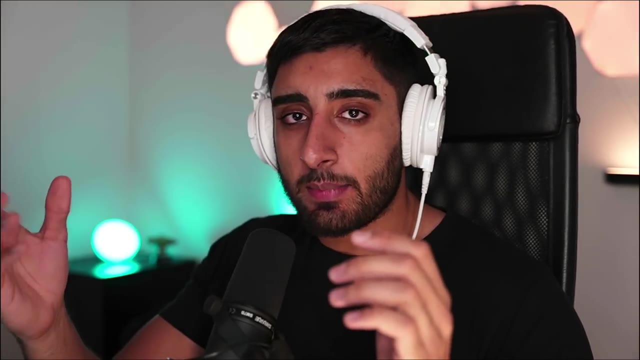 and why they make React so damn useful. Now, it's the reason why components can be reusable in the first place. So props simply stands for properties. And imagine we had an app like: imagine we had a component like a product. right, A product would have something like a name, a description, a price. 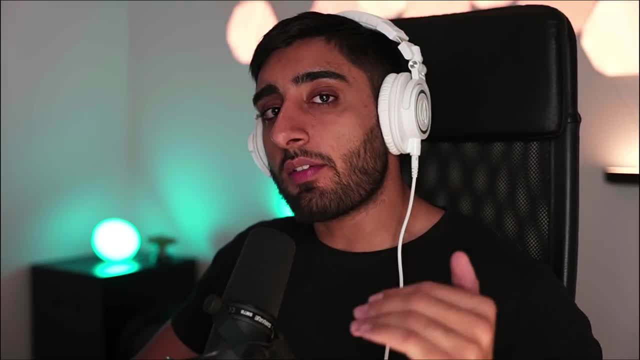 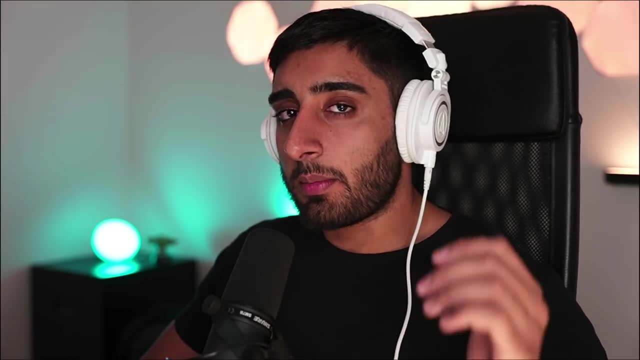 We would write the component once, and then we would reuse it several times And simply change the props that we pass to it. This would then render out to be the desired outcome that we want. So I'm going to explain this and break this down. 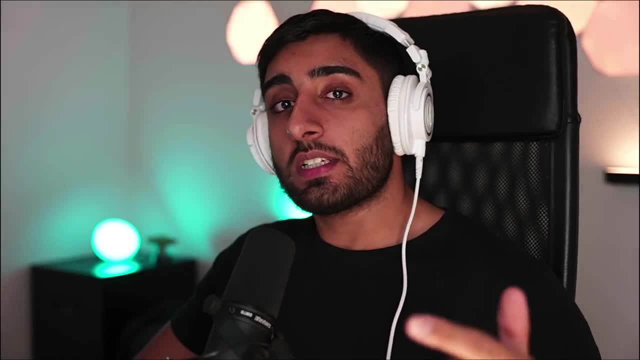 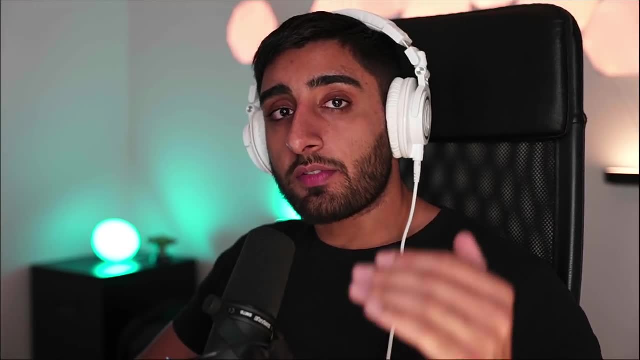 very, very simply for us. Now, it's worth mentioning that props are present in both functional and class-based components, So something we need to know is that props are passed from the top down. So imagine we had the app component at the top and then we rendered several products. 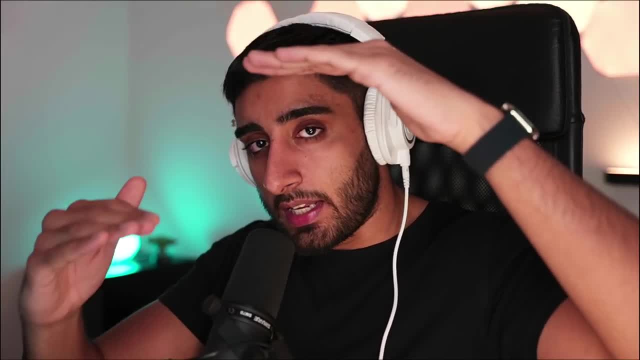 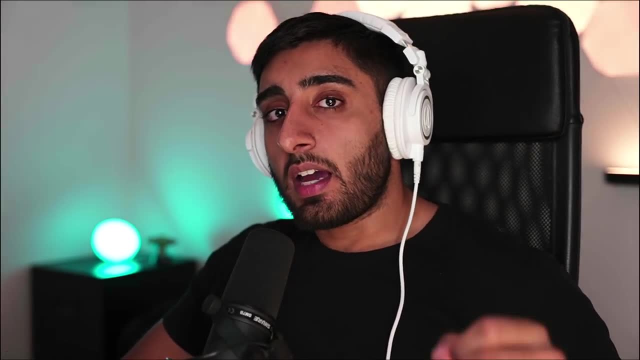 underneath. We would pass data from the top component down to those products and that would render out onto the screen. We would then be able to render out several components underneath that and pass props as required. This is why we have a tree-like structure in React and it's essentially 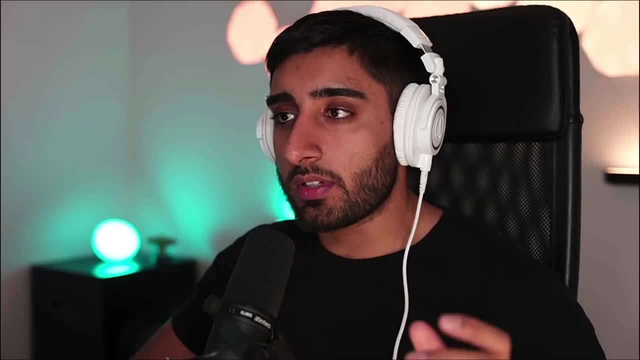 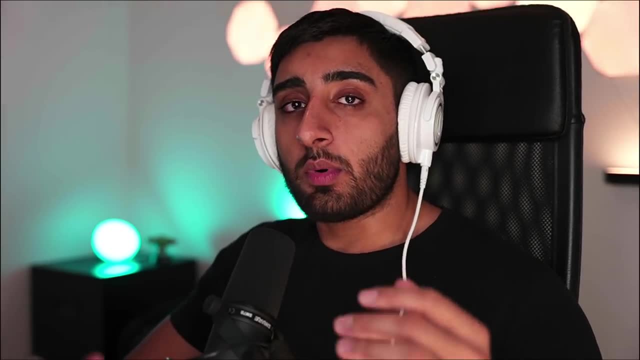 how React determines what to re-render at what different time. Now I'm going to go through an example here which will explain all of this to you, So don't worry if it doesn't make sense. We're going to use the example of a shop like Amazon, which is essentially an app, which has 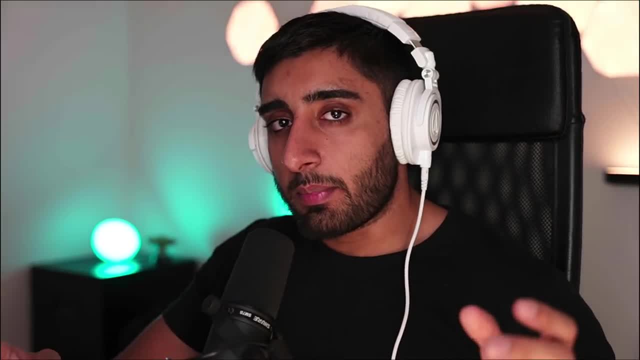 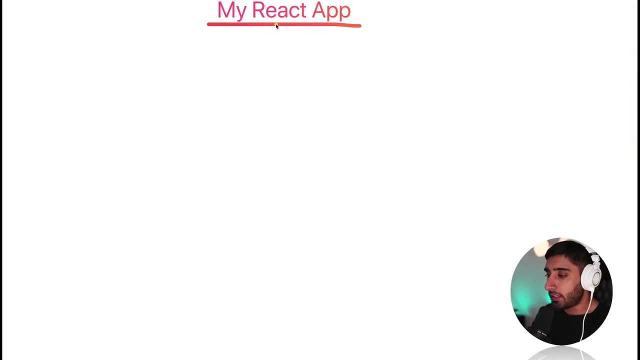 lots of different products on display and different sub-components are rendered underneath them. So let's dive into an example right now. So here is our application, and imagine it was an Amazon style app, right, So it's an e-commerce platform. Typically, we would start with the app itself. So 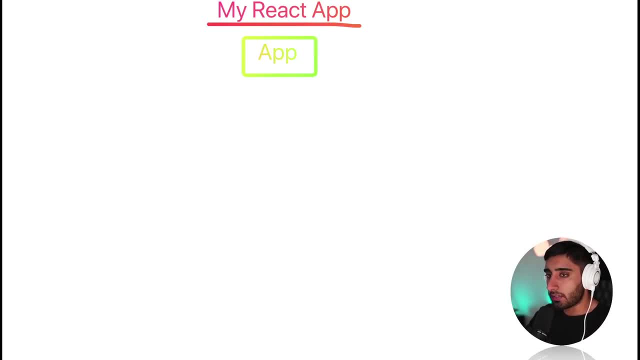 the app component itself. Just going to draw a little box around that to resemble a component. This would render out several sub-components beneath it. So imagine if it rendered out three product components. So we're going to go ahead and write the product over here like so, And what this? 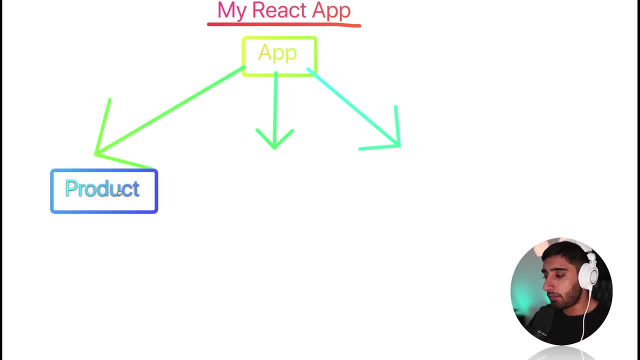 is we're going to go ahead and create one product and then reuse it several times where it's needed, okay, So this will actually pose several benefits. It means essentially we only write the code once and then we have styling for that one file. And if we ever change that, 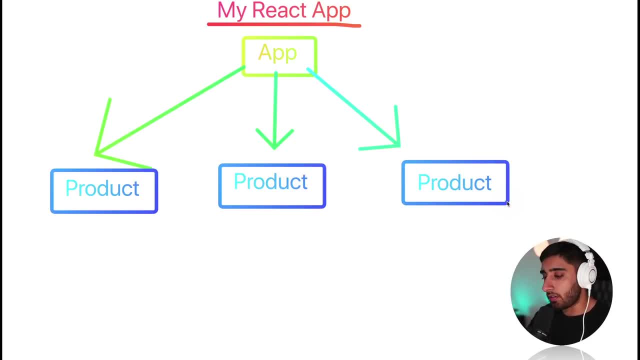 it's going to get changed in every single location that it's used across our app. Now each product can be customized via the use of props. So, like we said before, a product can have different properties, such as a name, a title, so a description. sorry, We can. 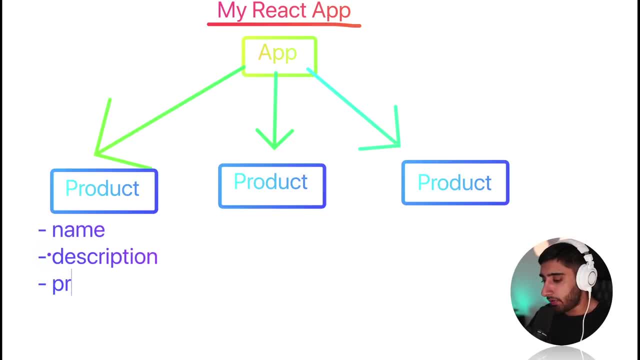 have a description and we could have something like the price right, And each one of these would get then passed over to each of the different components. So from the app component we would go ahead and pass the required props to each of the components. So, as we mentioned before, it would 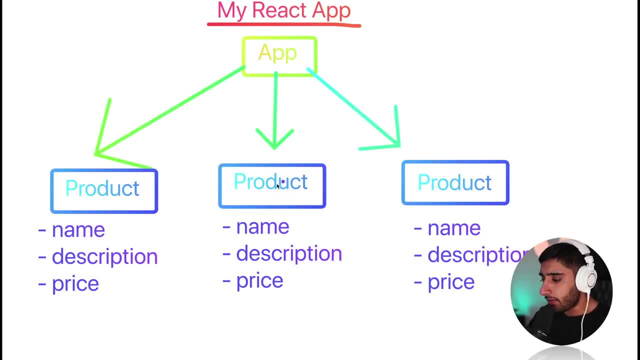 travel in a downwards, tree-like motion. Now, if we have a component beneath this level- so imagine a product has a item description component- So imagine a product has an item description component- then this would then get rendered beneath it as such. So imagine we could go ahead and do the following. So imagine the product went. 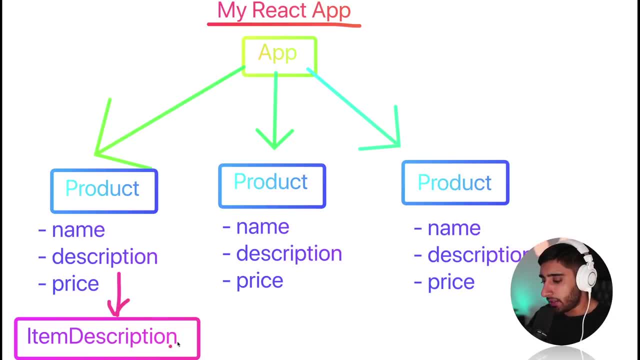 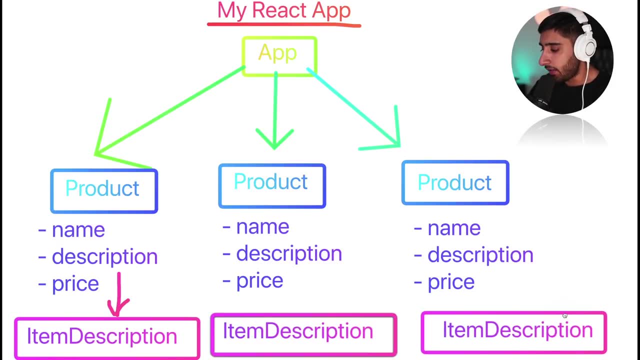 ahead and rendered this right here, and then we could go ahead and it could be rendered out again for this and again for this right. So, as you can see, we have a tree-like structure where it's simply components being reused over and over again. So this would render this and this would render. 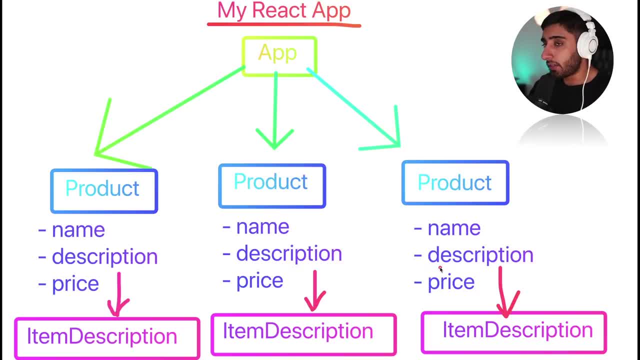 this And did you see that? So this is what we're going to do, So we're going to go ahead and pass that to each component. So the tree can go on and you can render whatever different components you want and however many different components you want at each level. Now, from this level, 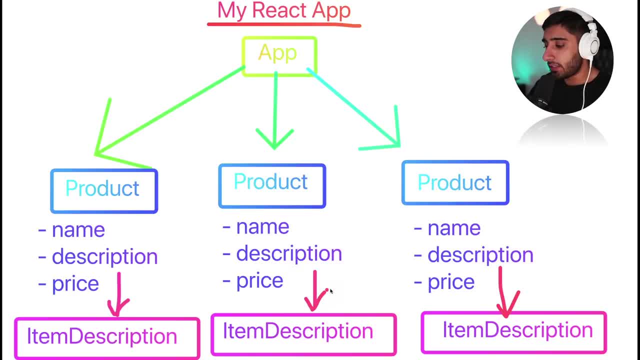 we could go ahead and pass something like, say, the item description only took things like the name and description, Then only these two can get passed down, if we only want that. So if we want these two as props, then they can only be the ones that get passed down, and we could maybe leave the 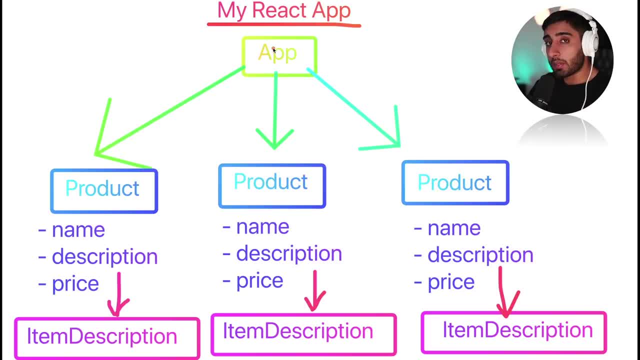 price, for example. So that is an example of how the props traveled downwards and were only downwards, so you can't actually go ahead and pass a prop back up the tree, okay. so it's a very important thing to know. now, another interesting tip that we have to remember are that props are 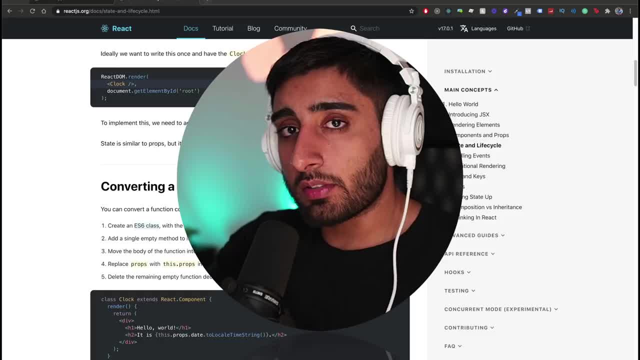 read only, which means once a component receives a bunch of props, they cannot be changed. we can only then use and consume the prop, but we cannot modify that property once it's passed down into a component. if we want to do that, what we would tend to do is use state at the component above. 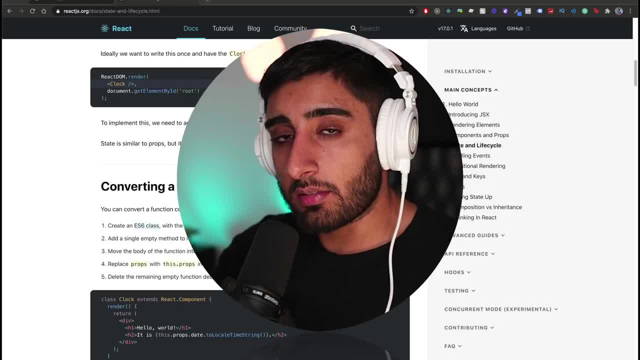 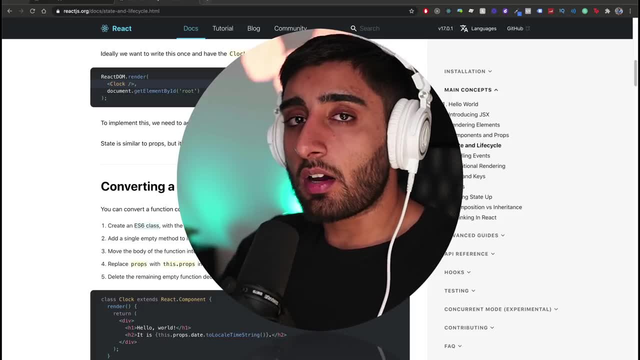 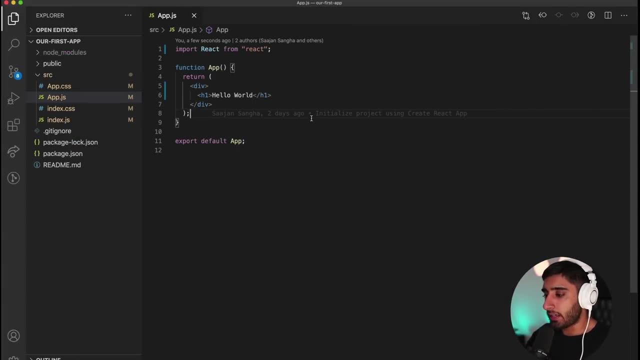 and then we would modify it accordingly and then pass it down to the child component. so what we're going to do now is we're going to dive into a demo application, so we're going to start off from where we left off. let's hop into our code. so here we have a starting application from create react app. 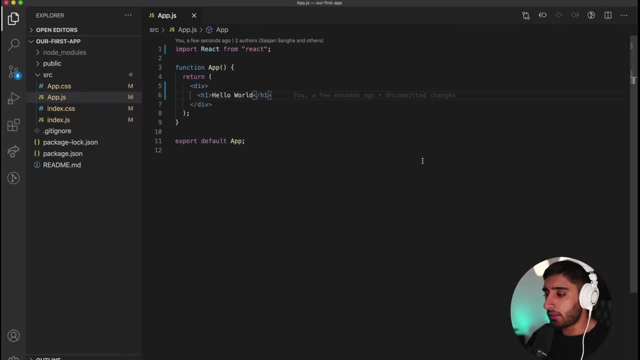 and we've just modified it to say hello world. now what we're going to do is we're going to go ahead and create our first amazon like application. okay, so imagine. what we're going to do here is we're actually going to go ahead and create a product. 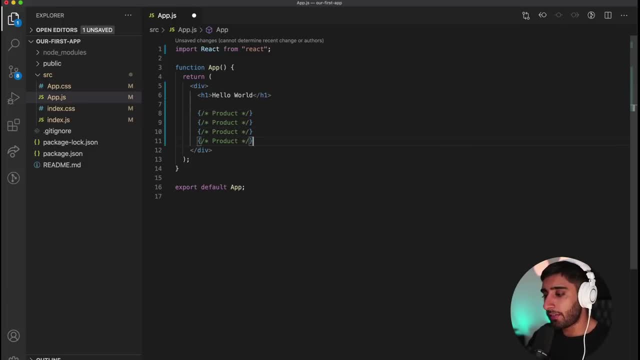 and then render it here, render it here, here, here. so we're going to have four different products and each one is going to take a name, a description and a price right. so imagine if we could pass these in each as different properties. then that would be pretty handy, because then we only have 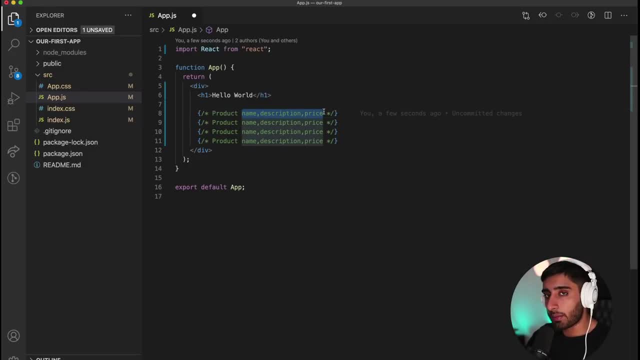 to write one component and we can reuse it by passing different properties to that component. so, in order to do that, i'm going to go ahead and create a productjs file and i'm going to use es snippets to go ahead and create my functional component. so here is our component. 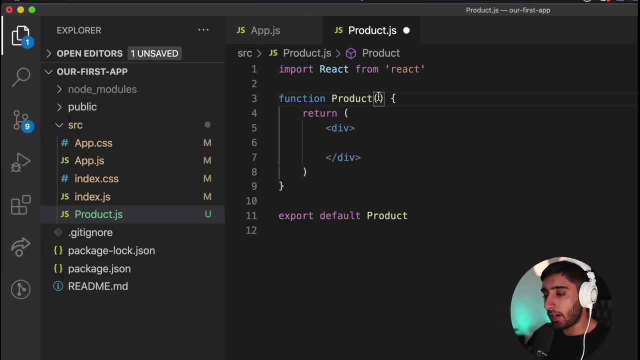 made. and what we're going to do at this point is right. here, where we have the product being initialized, we're going to go ahead and say props, so props actually get passed in as a parameter to a functional component or class-based component and the way we're going to access it. 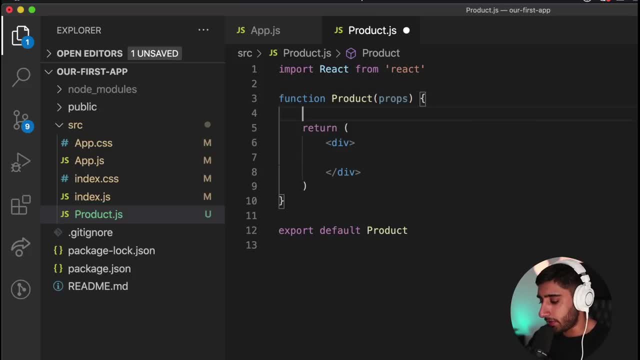 is simply by going ahead and doing the following. so we can go ahead and say props dot, whatever the prop is called. so if it was name, it will be propsname, if it was description, it'll be description, and if it was price, it would be propsprice. okay, so what we're going to do at 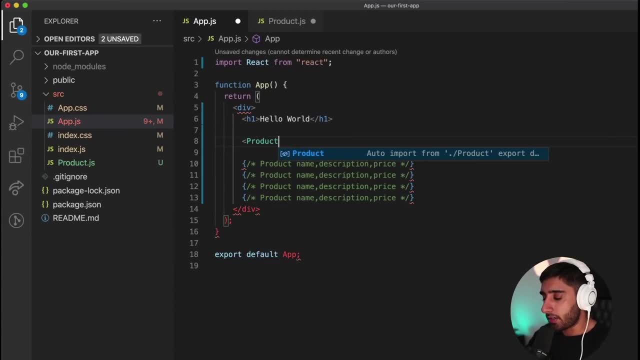 this point is: i'm going to go back here. i'm actually going to go ahead and render a product okay. so notice it says auto import. so you might get that sometimes with intellisense, but if you don't, you can go ahead and simply import at the top manually. now what we're going to do is i'm 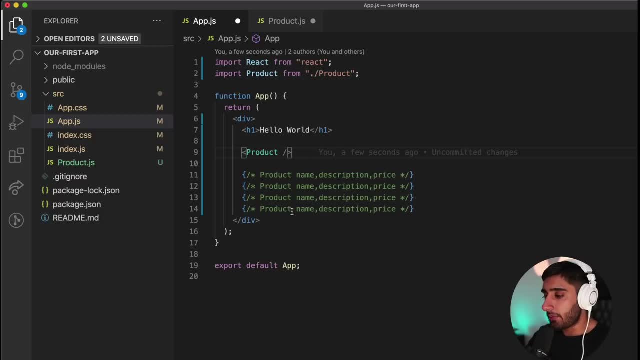 going to pass in three props. and props are passed in just like html attributes. so here i'm going to go ahead and say name, and for this product we're going to say amazon, echo, right. and for the description i'm going to go ahead and say um, your. 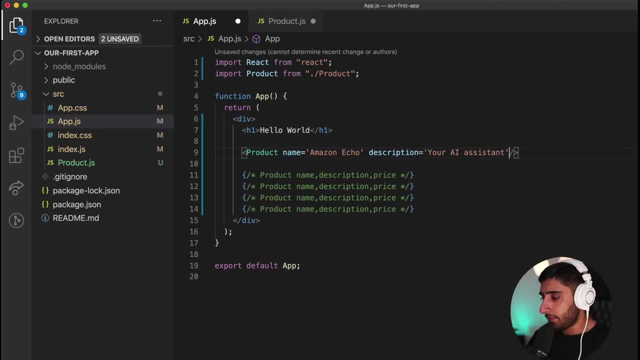 ai assistant, awesome, okay. and then for the price: i'm going to go ahead and pass in a value. so if we pass in a number, we do the jsx curly braces and i'm going to go ahead and say this is 59.99, okay, so there we go, that we have our first product with three different props being passed to it. so you, 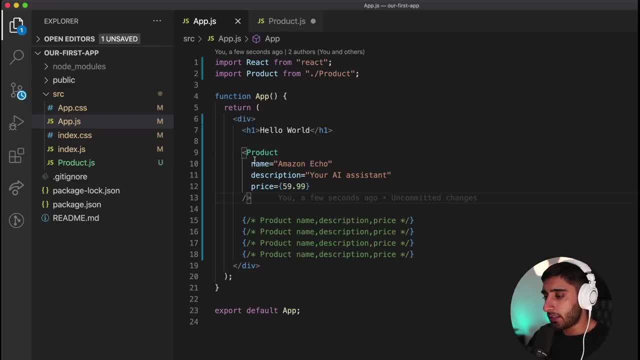 can see it's very clean syntax. i'm going to go ahead, save that file and the prettier did a nice job of cleaning that up. i'm going to go back to product and now we want to consume that information. so, firstly, i'm going to go ahead and say i'm going to go ahead and say i'm going to go ahead and say 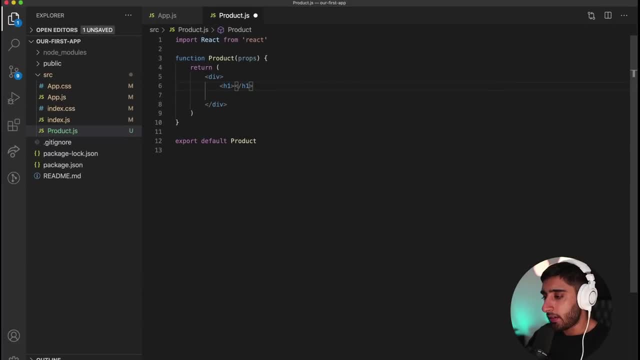 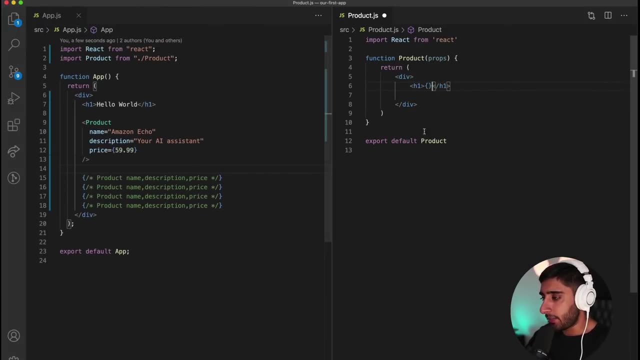 add a h1 tag. now for the h1 tag, i'm going to go ahead, firstly, make myself a bit more visible by having the app on the left hand side and the product component on the right hand side. so here i'm going to go ahead and use the name prop. so i'm going to say propsname as a h1. 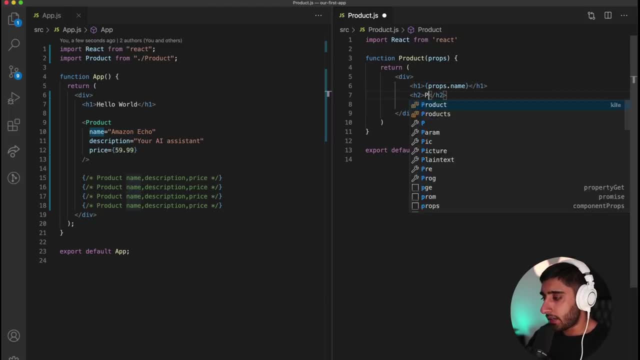 tag. right then, as a smaller h2 tag, i'm going to go ahead and say propsdescription, okay, save it now the price. i want to go ahead and say propsdescription and i'm going to go ahead and say: want to do something special. I'm going to go ahead and say we have a h3 and I'm going to go ahead and 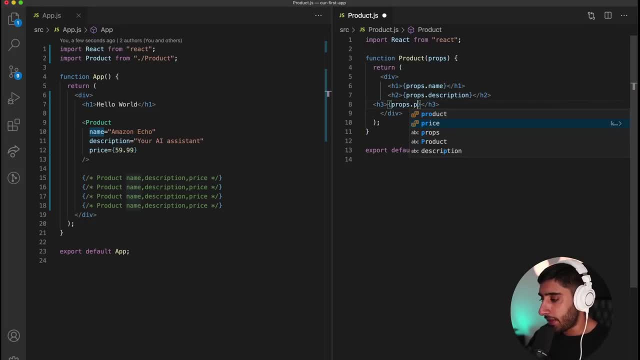 add in the props dot price here. but what I'm going to actually do is I'm going to go here, I'm going to add in the dollar sign before it, because it's going to be resembling a dollar amount, right? so we're going to have props name, props description, props price. so let's go ahead and test this. I'm. 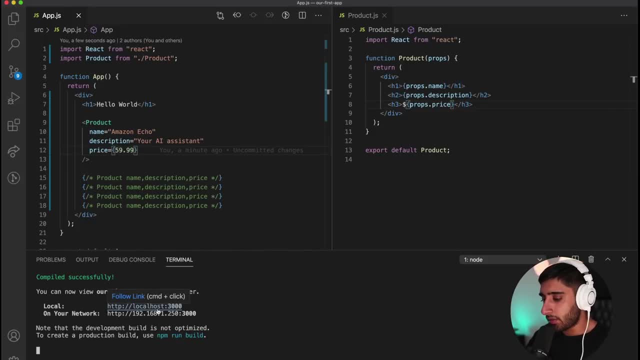 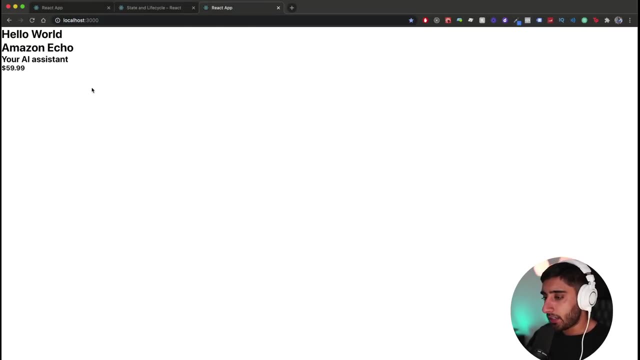 going to go ahead and press command j, pull up my terminal and we are running on localhost 3000. I'm going to go ahead and open this up right now. so let's go over to localhost 3000 and you should be able to see. there we go. we have our component being rendered on the screen so you can see it. 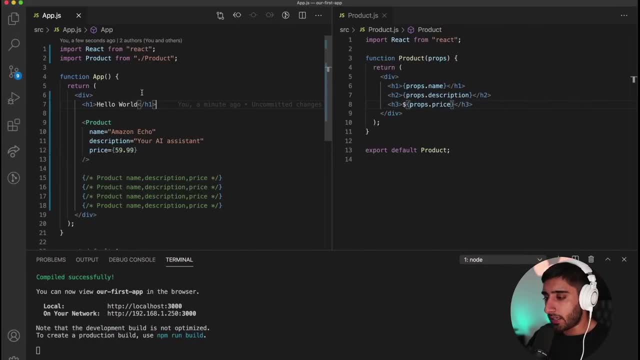 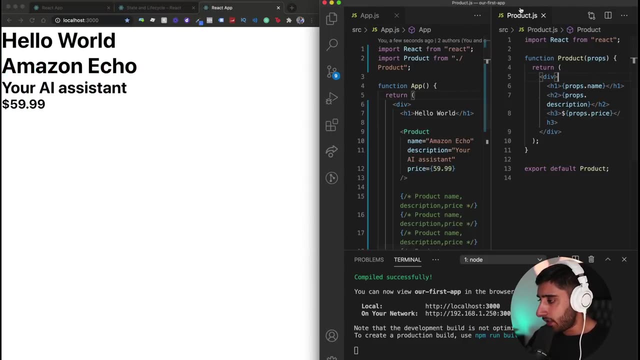 actually pulled through that property that I passed in. so let's go back and jump to our code, and what I'm going to do is split the screen for you guys so you guys can see this very, very simply, and what I'm going to do now is pass over here. so here you can see an app. we have the product. 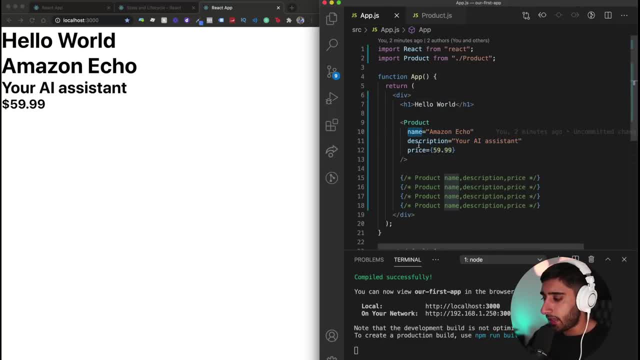 being rendered. we have the name amazon echo, we have the description, your ai assistant and we have the price: 59.99. okay, now what i'm going to do is i'm going to change the name, to go ahead and prove that this is correct. we're going to say google. 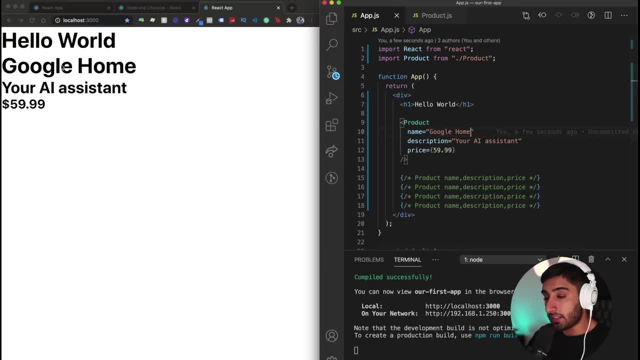 home and i'm going to save, and now you can see it changed google home. so this is really handy. and what is this handy for? it means that we can actually go ahead and make one component reuse it several times all throughout our application. so what i'm going to do now is i'm going to come copy. 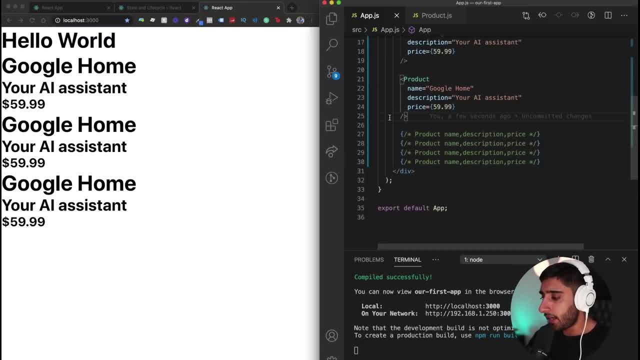 this. i'm going to paste it three times and i'm going to get rid of these comments, okay, and i'm going to change each of these products. i'm going to say iphone and i'm going to say the new iphone 12 pro max, nice. i'm going to say the best iphone, because that's what they always say, and i'm going 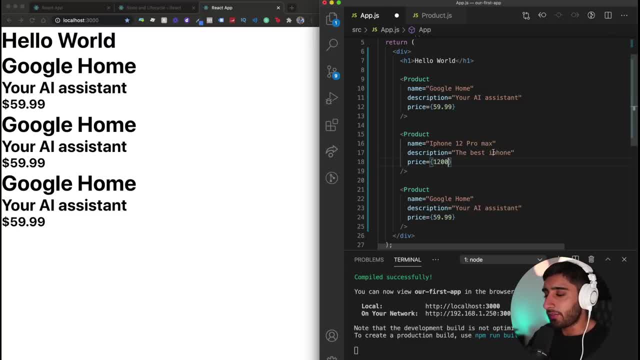 to say: price is 1200 because you know iphones are expensive. and then here i'm going to go ahead- and this was bugging me, i can't do that to myself all right now. here i'm going to go ahead and say: let's go with a macbook pro, okay. and then your favorite computer, little pc attack, right and 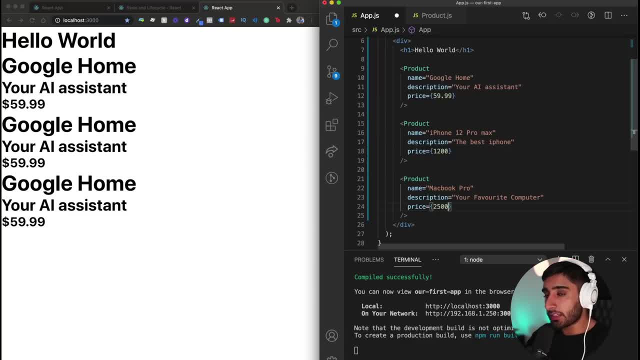 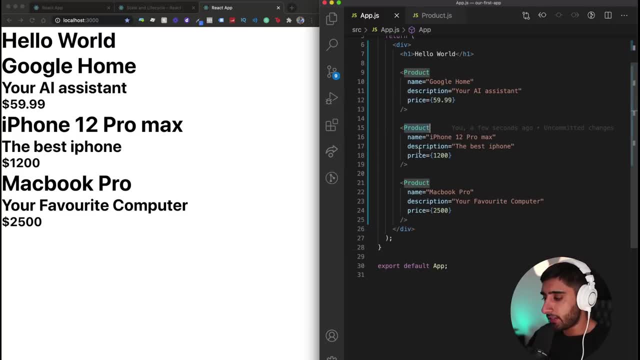 then we're going to here, we're going to go ahead and say: it's 2500 because they're even more expensive, right? so i'm going to go ahead, save it and watch the magic. there we go, guys. so you can see, we're just reusing this component three times with different props, properties. right, and it goes. 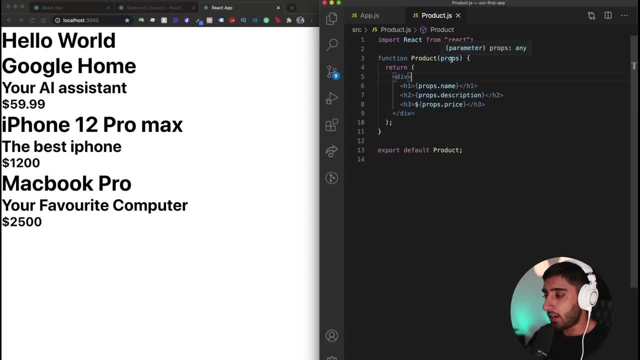 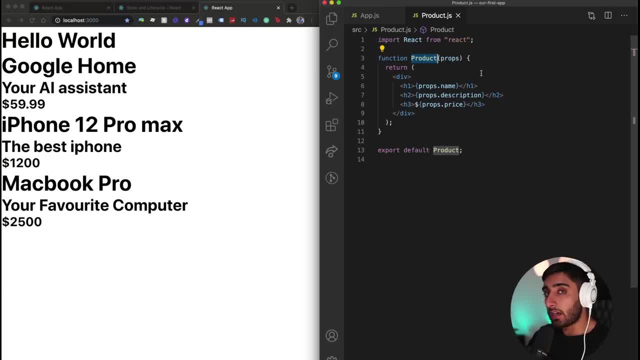 child component underneath this and pass the props down to them. so the first thing i'm going to do is show you a little neat trick. so in es6 we have something called es6 destructuring. so what we can do is props. instead of saying propsname, propsdescription, propsprice, we can have curly. 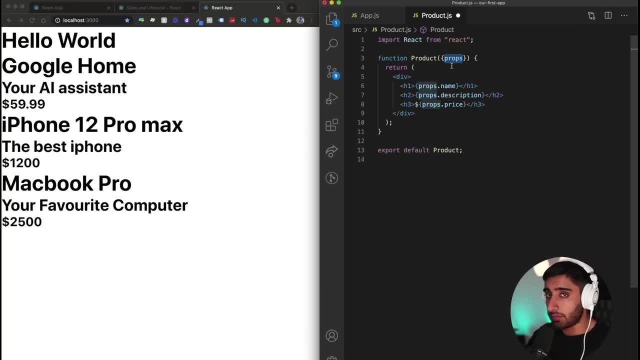 braces around the props to say: pull apart this product, and then we're going to go ahead and destruct this object, which is called destructuring, and then what we can do is we can go ahead and grab the elements directly at this point so we can say description, prop and price. so now what i can. 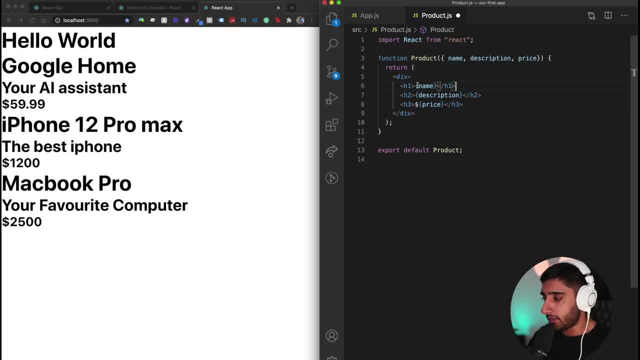 do is i can go ahead and get rid of all of the following things. so now it's name, description and price, because we're actually pulling apart the props at this point, destructuring it, and then we're rendering it. so you can see if i save it. nothing broke okay. but if it broke at that point, 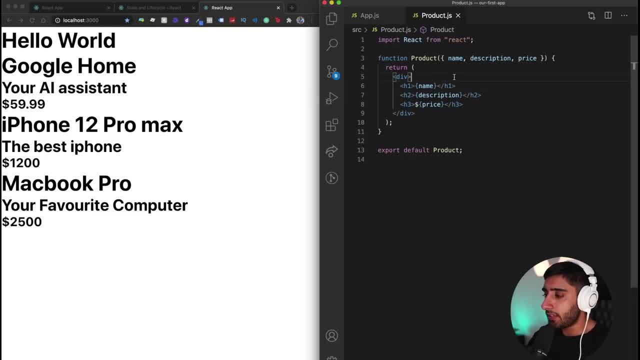 probably didn't have some of your syntax right. so what we're going to do now is i'm going to create a subcomponent called item description and we're going to pass props down to that one and i'm going to show you how that tree structure works. so let's go ahead and create a item description component. 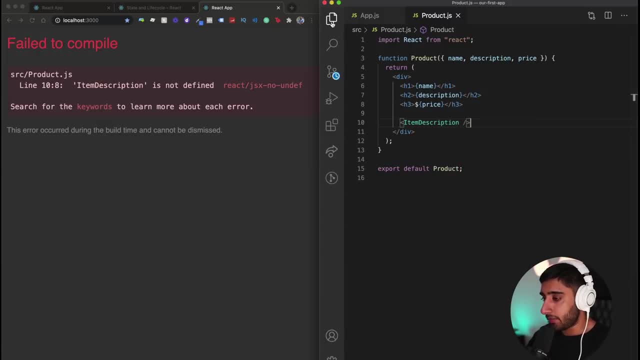 and this will most likely error, because we haven't got an item description component, which makes sense. i'm going to go ahead and create that item descriptionjs, save it, and i'll go ahead and say: rfce, boom, we have it up and running. okay, so that's awesome. and then now we go ahead and we get some. 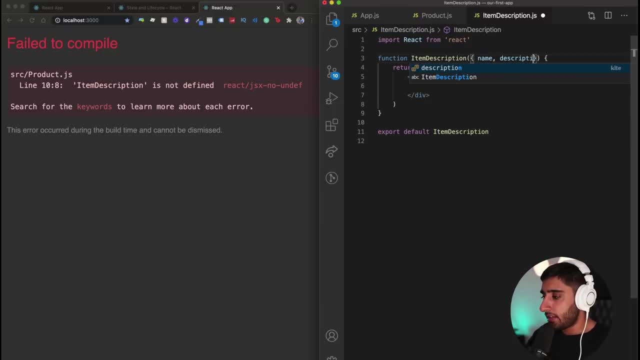 the item description is going to take the name and the description only. okay, so just a sort of test right here. so let's go ahead and save that. and then what we're going to say is: it's going to have a p tag- oops, a p tag- which will then show the name. so let's go ahead and say it takes the name. 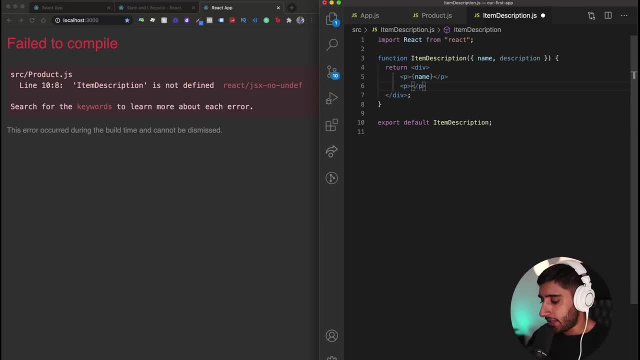 and i'm going to have another p tag underneath it which is going to be in italics, and this is going to have the description. okay, there we go. and now what we're going to do is we're going to go back to our product, we're going to go to the end of the component name control space bar, neat. 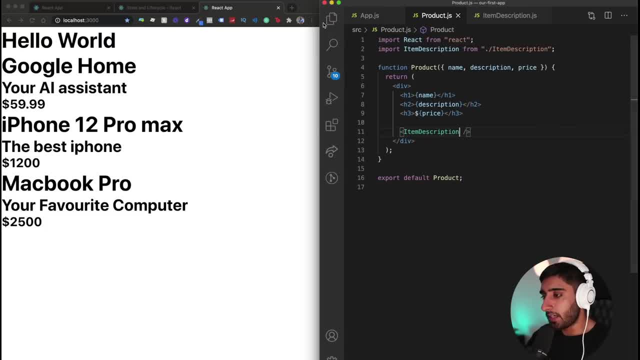 little trick: auto import. that will be a nice little trick for you guys. and now what we can see is the item description renders, but i can't see anything on the screen. sonny, that's correct, because we haven't actually passed any props, which means that this is actually blank, right? so what? 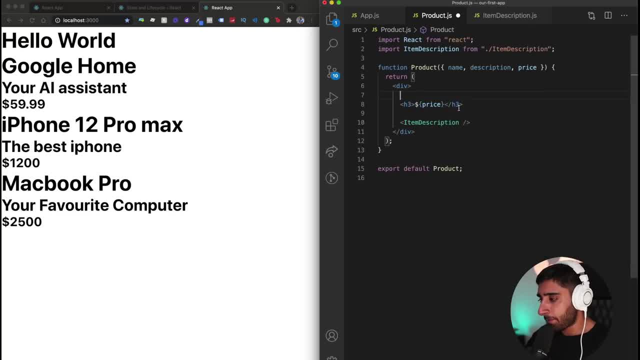 i'm going to do now is, rather than having the name and description over here, i'm going to go ahead and say i'm going to move the price underneath the item description as such and i'm just going to simply pass this down as a prop. so i'm going to say the name prop in this case is the name prop that we passed. 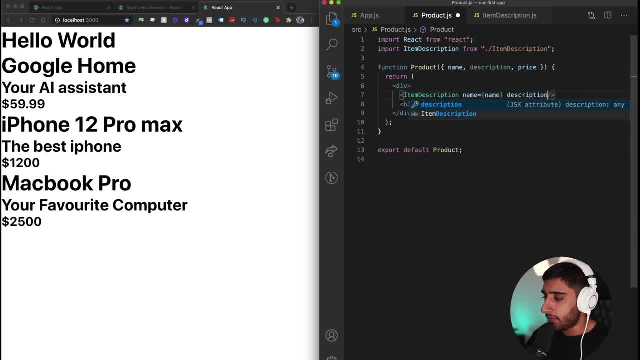 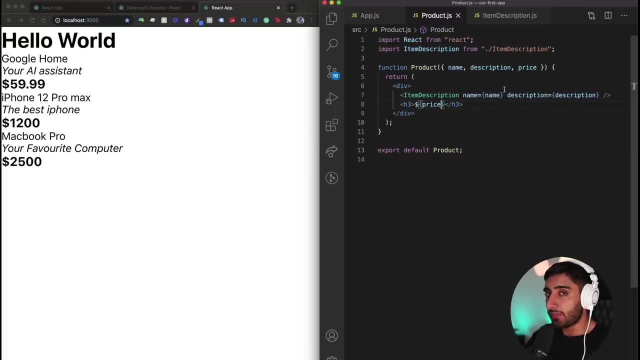 down from the app component, and then here i'm going to say the description prop of im description is the description prop passed down from the app. and then here we keep the price in this level, save it, and now you can see we have a nice item description with a big price, right. so it's very. 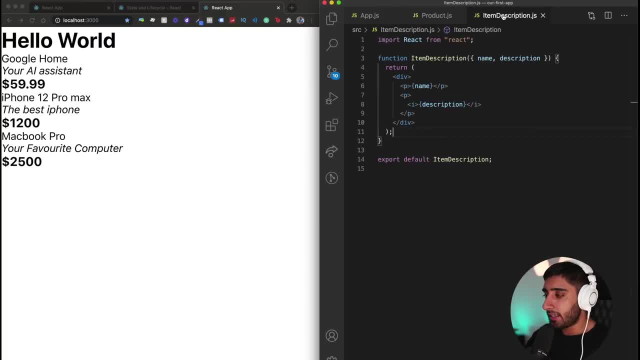 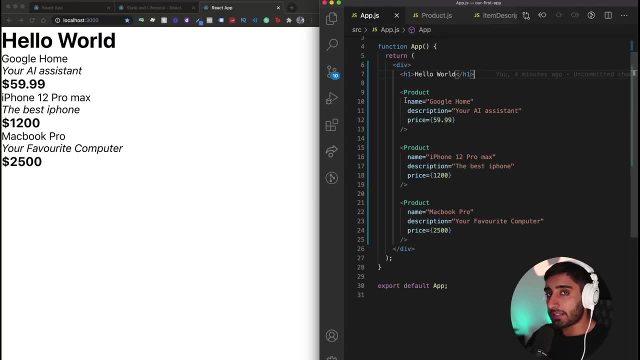 very powerful. okay now, this is extremely reusable. it's extremely powerful and it's quite simple in terms of how effective and use useful is. so notice how- remember i said it was top down, which meant that you can't pass the prop back up. so if i want to push the name back up to the app from this level, 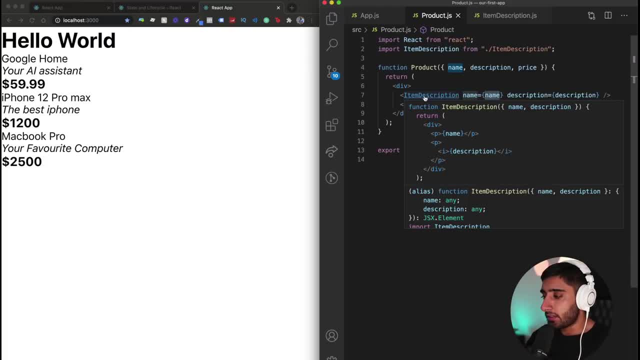 we can't because we went downwards and again, if i was go inside the item description, i can no longer pass the name and description back up. okay, unless we introduce something like redux, in which case there's a whole different type of data flow, which we're going to talk about in a later lesson. so 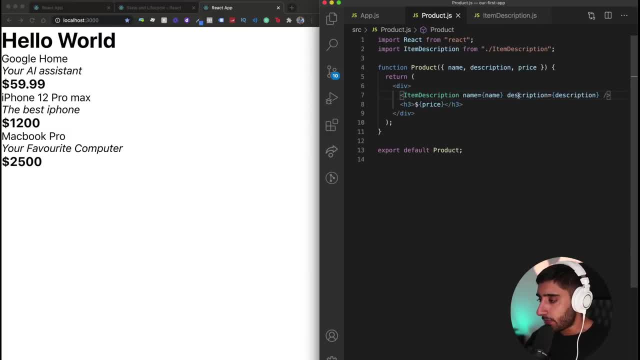 with that said, now what we're going to do is we are going to go ahead and pass the name back up to to demonstrate how you can change one of these components to a class-based component, and that is going to show you, guys, how to use props inside of a class-based component and show you how it's. 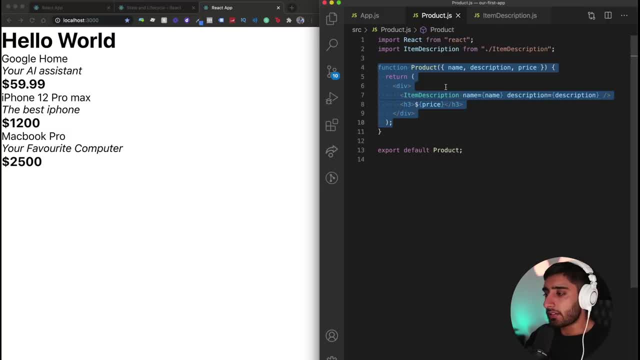 a little bit more complicated to write that. so, as i've mentioned previously, functional components are the way forward. however, it's most likely that the code bases that you're going to be interacting with are older, and remember, guys, class-based components were out longer than functional components, so we need to know both. unfortunately, 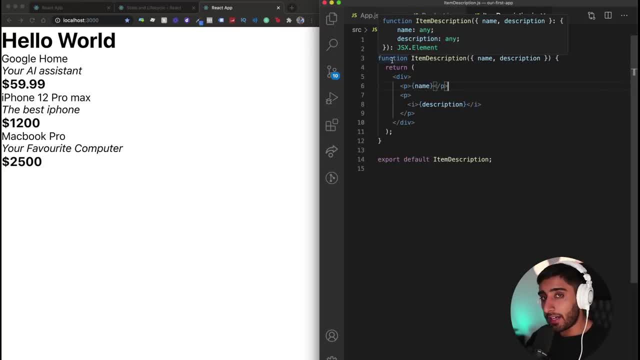 it is just the way it is. so at this point, what i'm going to do is i'm going to refactor this to become a class-based component, so that way you get some experience about going from functional to class-based as well. so at this point, what i'm going to do is i'm going to go ahead and copy this. 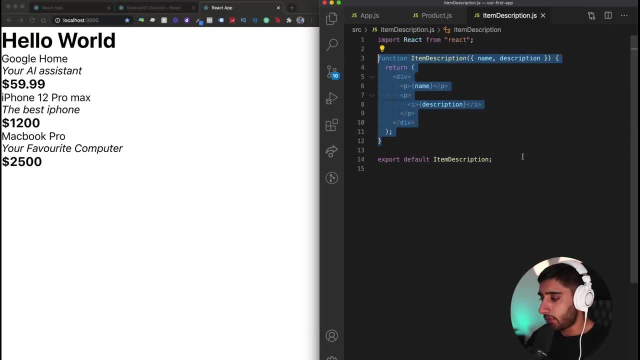 jsx, so i don't lose that for later. i'm going to go ahead, get rid of all of this code and i'm going to use my handy little snippets rcc to create a class component. now, inside, i'm going to paste back my jsx so we have everything we started with. but remember, don't actually have access to my props. 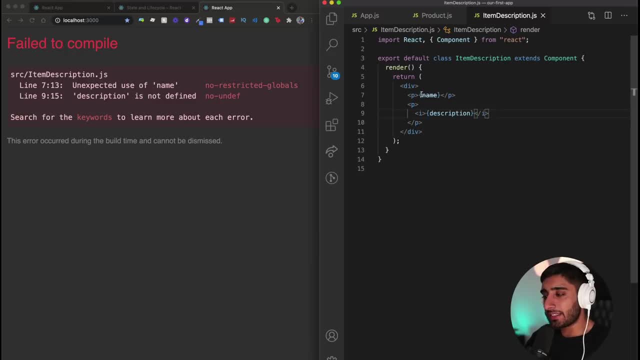 i use the props. so in class-based components it's not actually as clear as it may have been before. so firstly we need to go ahead and say this: dot, props, dot name: now right. so again it's a little bit more abstracted. and even here i need to say this: dot, props, dot description, hit save and you. 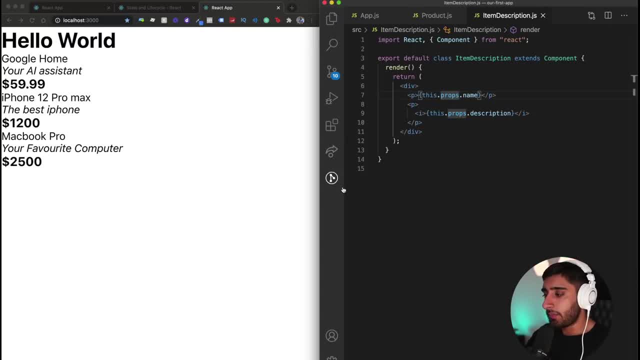 can see, now we get access to those props right. so you can see, this is actually a bit more. there's a bit more code going on. right, we have the class, we have the extends component, we have a render and then we have the return block inside of it. okay, now what you might see in traditional 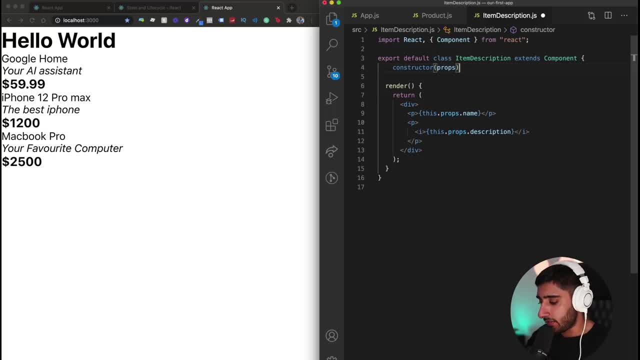 apps is. we used to have to write this syntax like so, where it said constructor props, super props, but we no longer actually need to go ahead and write this, and this is typically where we would go ahead and say this dot state and define our state. if we were doing so, as we showed you in 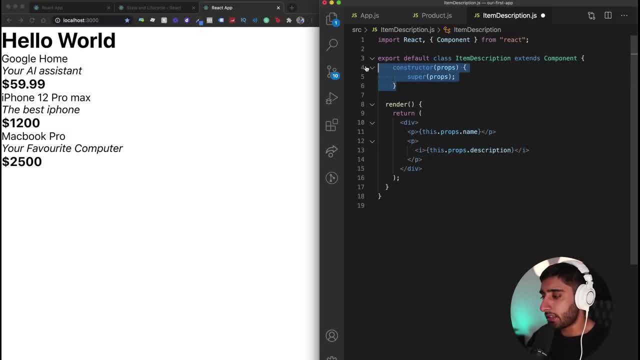 the previous lesson. okay, but in the modern react syntax we don't actually need that, which is quite nice. okay, and you can see it still works without that. now a little trick and one of the little top tips i've actually found people do. now what we can do. 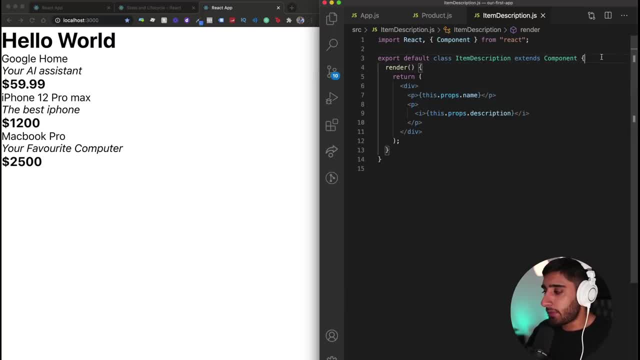 at this point to clean this up a little bit: if you are stuck with using class-based components is inside the render block where we can actually have some jsx. we can go ahead and say this, we can go ahead and say const and then we can destructure, so object destructuring in another es6 function. 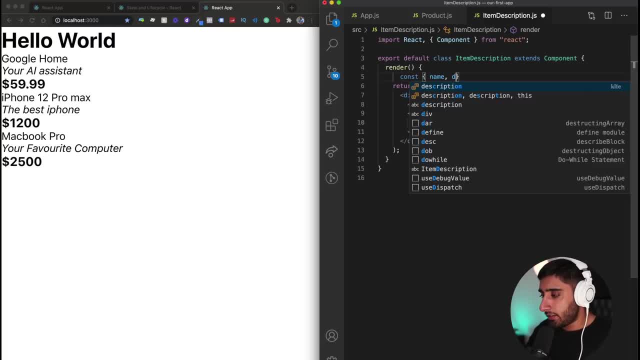 is, we can go ahead and say the name and description from this dot props and what this is doing is going inside of this dot props and it's pulling the name and description. so what we can now do is go to this dot props and get rid of it. so that's another way of cleaning up your code. if 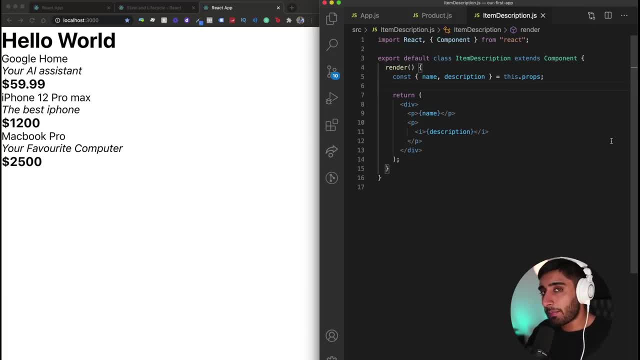 you're stuck with using a class-based component. but remember, guys, you're not going to be stuck. it is always possible to go ahead and translate this entire code right here, to a functional component. so, with that said, guys, i hope this has been useful to show you the differences between a. 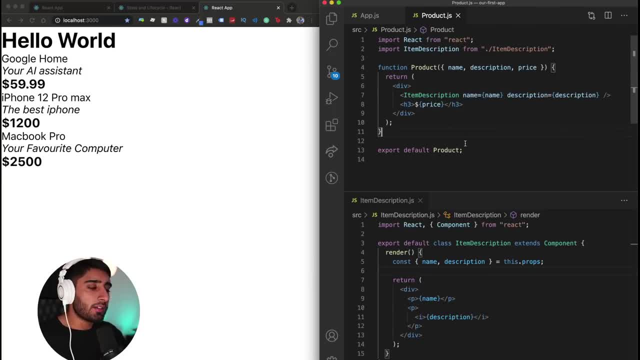 class-based component and a functional component, and hopefully you guys are on my side and you prefer the functional approach, because that is the modern approach for many reasons, and the main one being simplicity. guys, use that one. it's a lot more simple and with that said, guys, it's very clear how we can go ahead and write code once, reuse it in several places with. 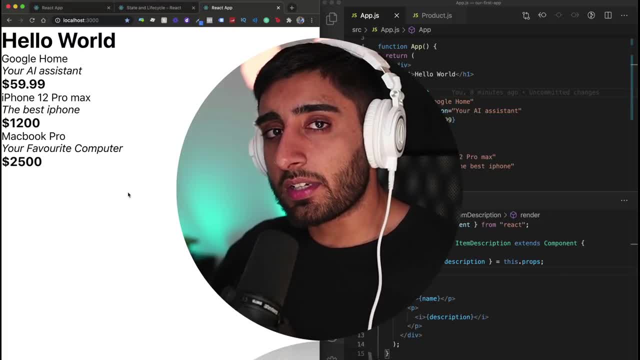 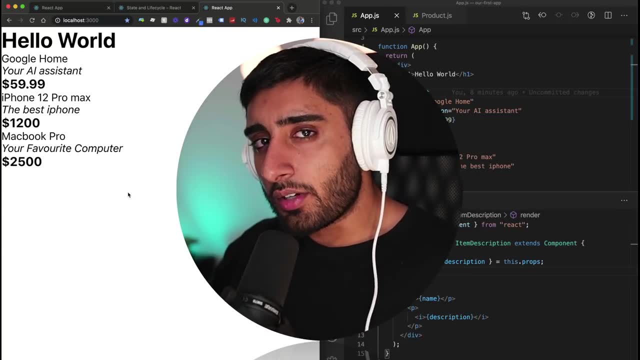 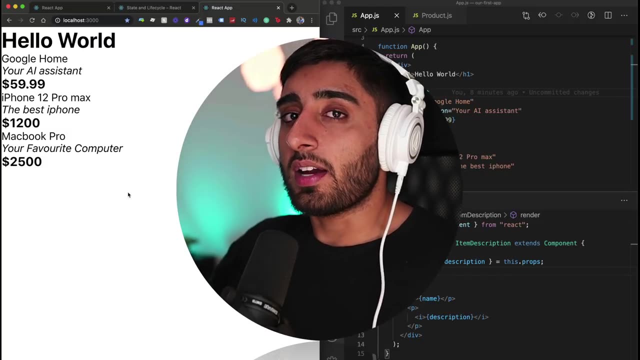 props now. this doesn't look too great. so in the next session i'm going to show you guys how to add some style to your code and actually style each of your components, and also show you how to level up your react skills by combining components with their own css files and watching the magic unfold in. 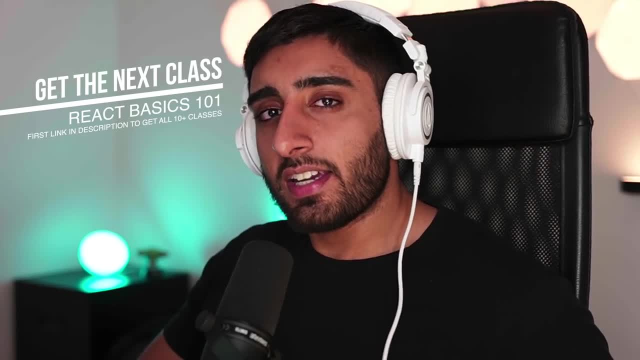 front of your eyes. so i hope you guys enjoyed that and i will see you guys in the next lesson. peace.